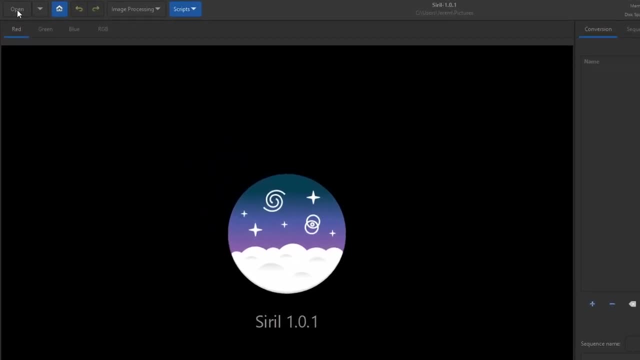 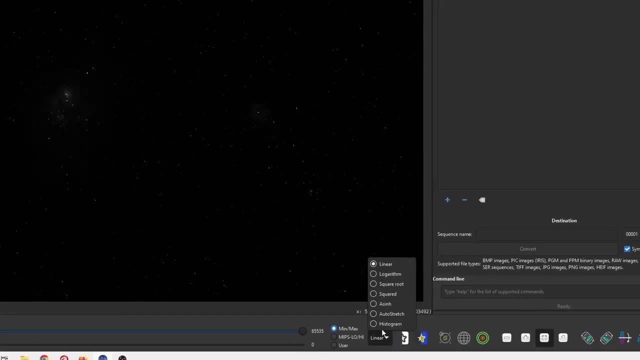 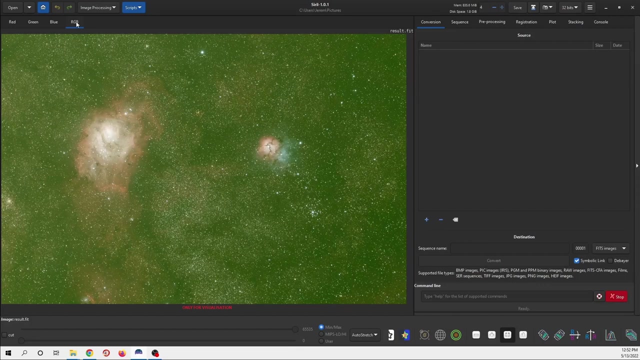 Let's begin with opening up the stacked photo. So let's go to the open and open up the stacked file. This is how the picture should look like. First let's change from linear mode to auto stretch mode. Then let's change the view from monochrome to RGB to have a peek. 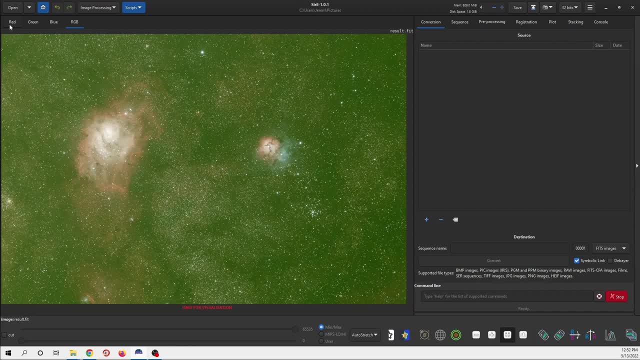 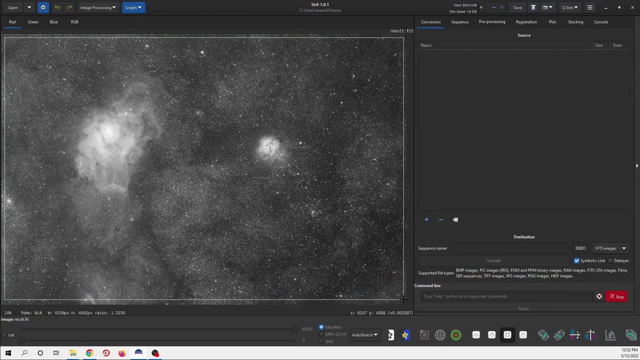 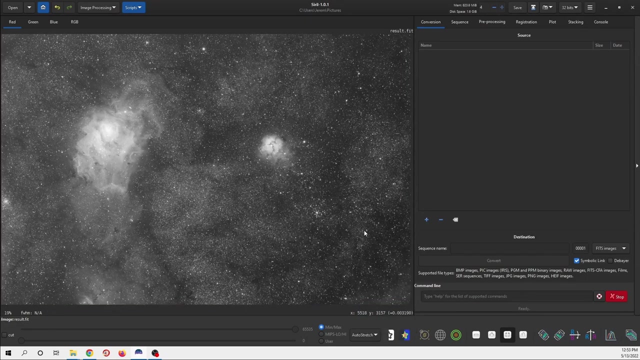 at the data. The green tint is normal at this stage. We will do colour correction later. Let's begin processing by first cropping the image. This step is very important because the edges of the photo often have weird artefacts. Next we want to remove the gradient To do this. go to image processing background. 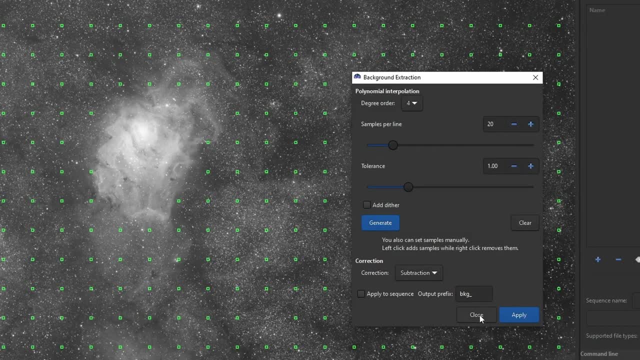 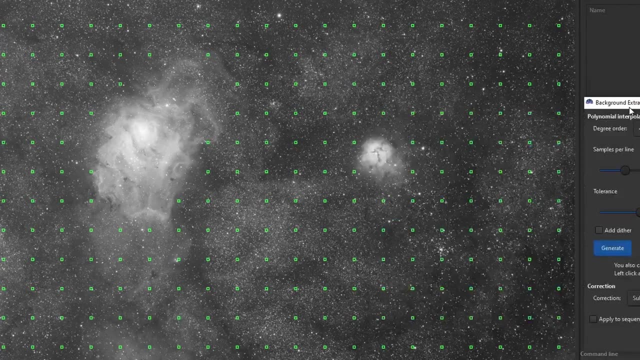 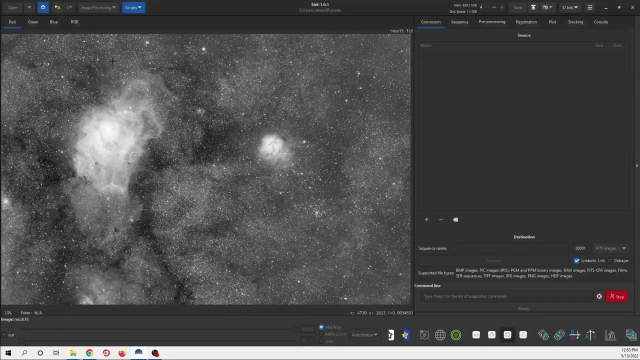 extraction: click generate. Now you will see small green squares throughout the image That will be used to compute a gradient. If any of those green squares are on Nebula, make sure to remove it. Click apply. Now we want to fix the colour. To do that, we will. 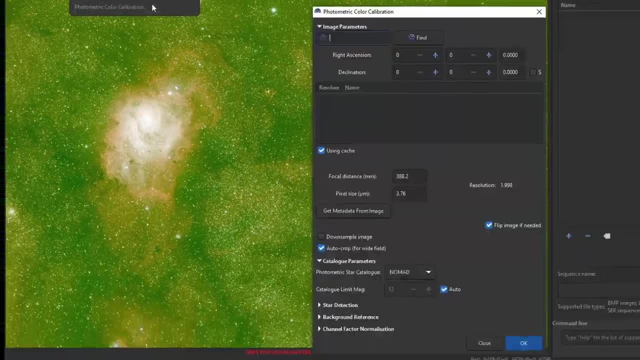 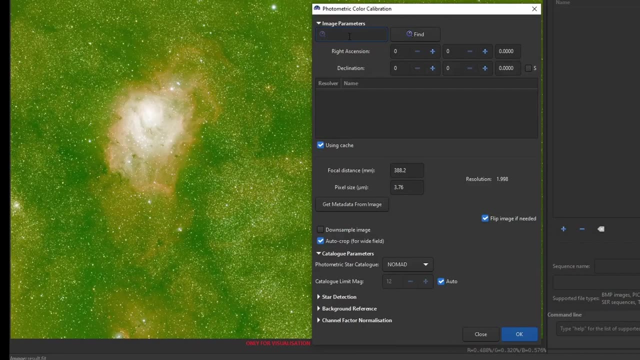 go to colour collaboration And then photometric colour collaboration. By the way, you must be connected to the internet to use this feature. Type m8 in the image parameters and click find. Click Lagoon Nebula and then you want to add correct focal distance and pixel size information Often clicking. 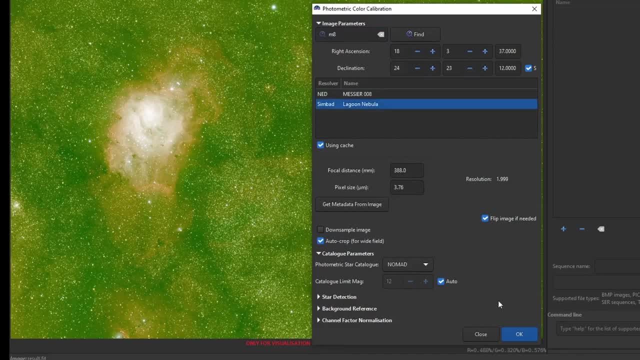 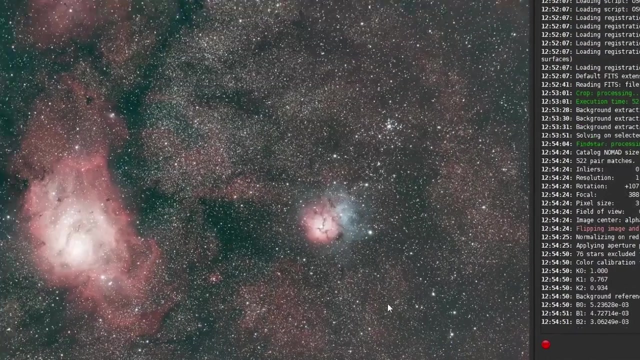 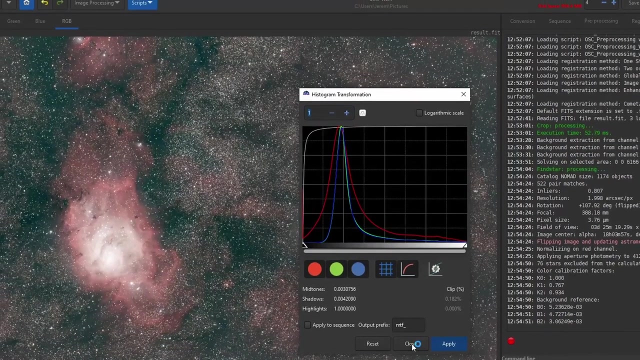 get major data from image automatically fills this. If it doesn't work for you, just type manually, Click OK. Next we will perform an auto stretch to this image. To do that, let's go back to linear mode and then image processing, histogram transformation, auto stretch apply Again. 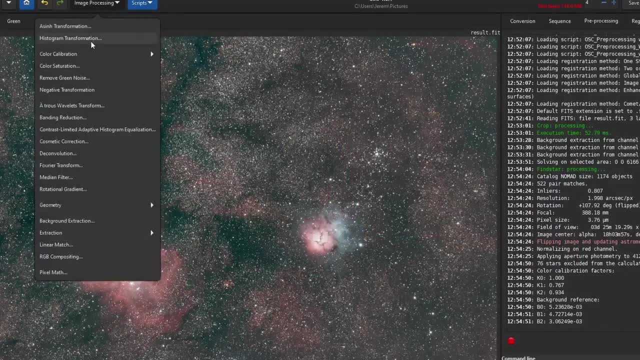 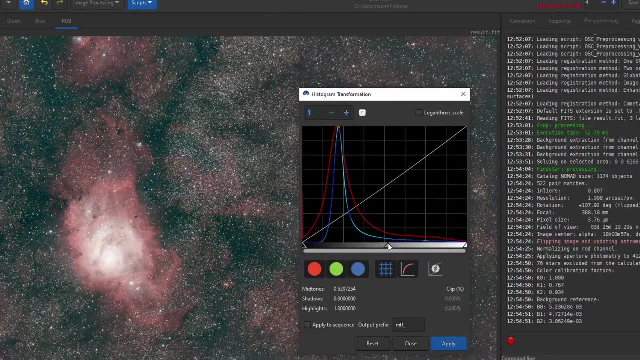 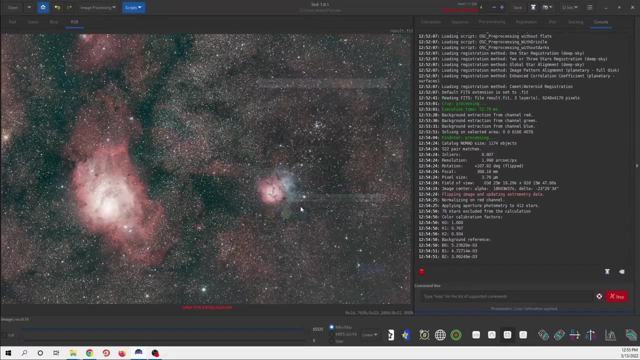 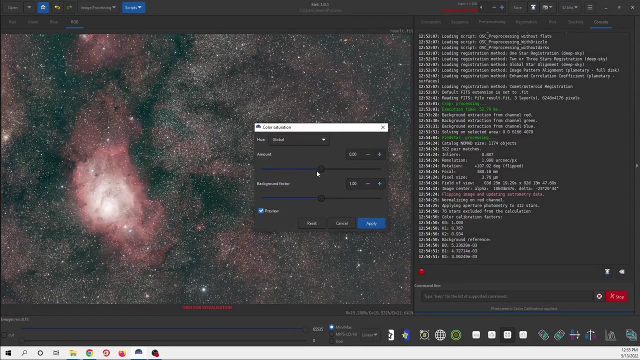 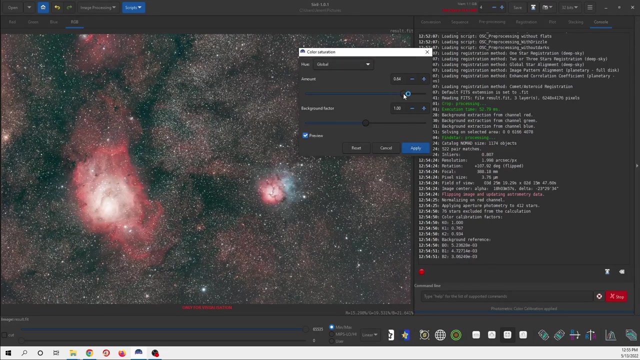 go to histogram transformation and then make fine adjustments with the slider. We want to focus on colour saturation next, So go to image processing, colour saturation, and feel free to experiment with different levels. This photo looks fine to me. You can do more edits in Photoshop if you like, but I am happy. 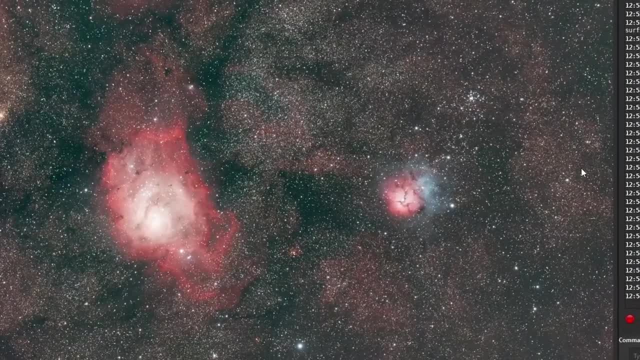 with how this looks. If you found this to be helpful, please subscribe.